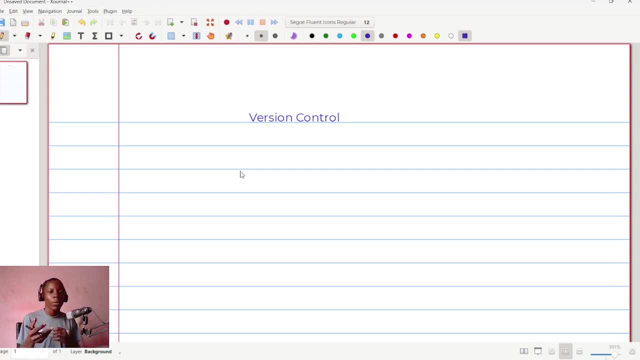 let me ask you a simple question: What version of the phone are you using? Alright, so, is it an android phone? If it is an android phone, what version of the android phone are you using? or what version of the ios phone are you using, or even the various applications that you use? So, 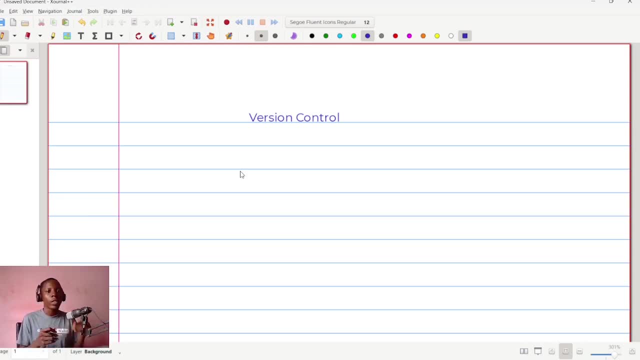 even youtube that you're using to watch this video. what version of youtube have you installed Now? does it click? Have you started thinking about it? the last time you downloaded whatsapp or any application, you could have been told or update to the newest version. but the question is: why do we? 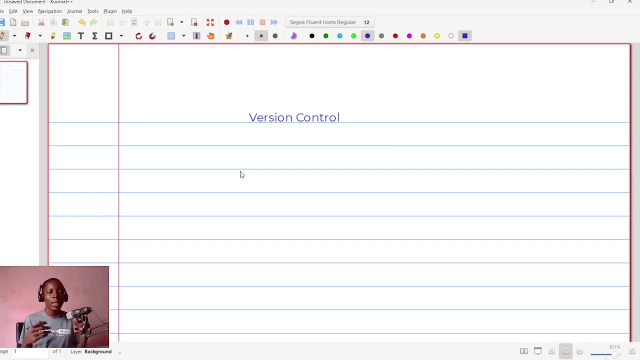 have all of these versions coming up, and what is a version in the first place? So, basically, when you talk about a version of any product, now, remember that we are dealing with software engineering, so I'll focus the narrative around software engineering. when you talk about a version of a software, it's a. different term. What is a version of a software? So essentially, what it means is that you are creating a copy of an existing um- I would have used version in this case- but an existing code. you are creating a copy of it or the software that you already have. you want to create a copy. 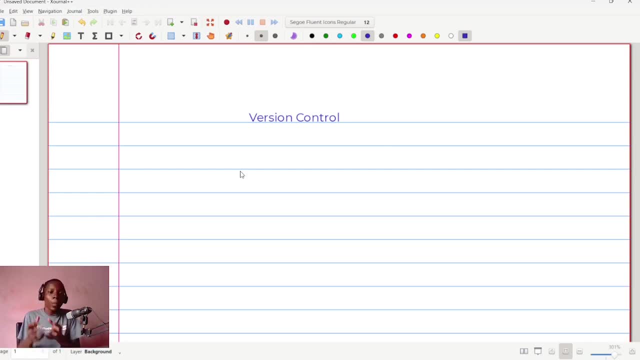 of the software, then you are also able to make some modification to the copied version or the copied form or the copied software. So essentially, when you talk about a version, a modified form of an existing substance, so for instance, if i take this case here and i want to create a version, say this is version zero. this is the very first version that i created. 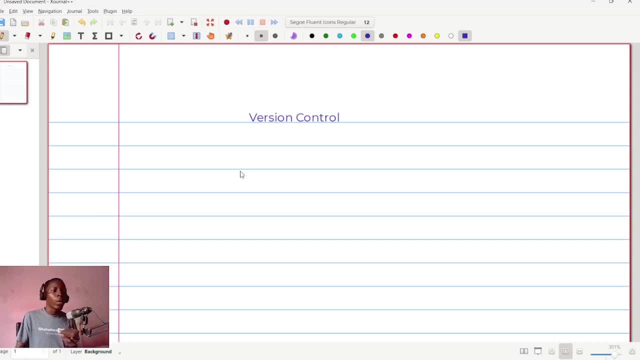 okay, the very first form of this is that i created. if i want to create another form, sometimes i'm not too sure whether the changes that i'm going to make is going to distort this, but i like this the way it is, so let me keep this over there and make a duplicate of it, or make a copy of it. 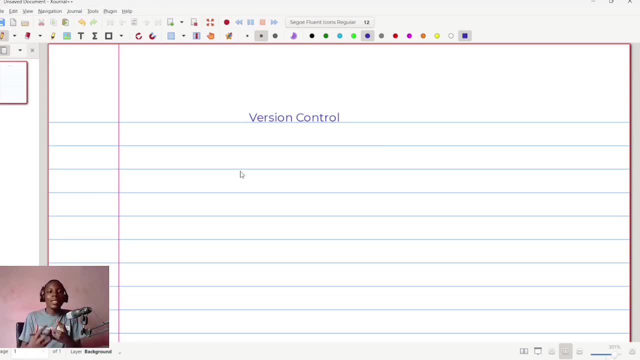 then i'll make the changes to that copy so that i can present that copy as a different form of this. so essentially when i come out of the product i'll still have this already there as version zero. then a new one that will come will be say version one. then the next time i can create another one. 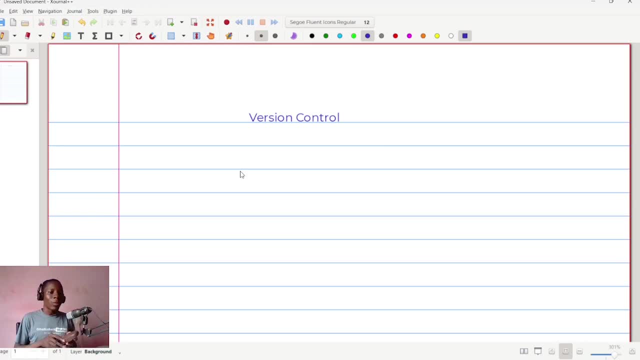 version two, version three. that means that at any point in time, we still have our access to the various versions, and this is essential in software development. along the line, you will come to appreciate why you need to be creating these versions, but i hope this makes sense. the concept of versions. 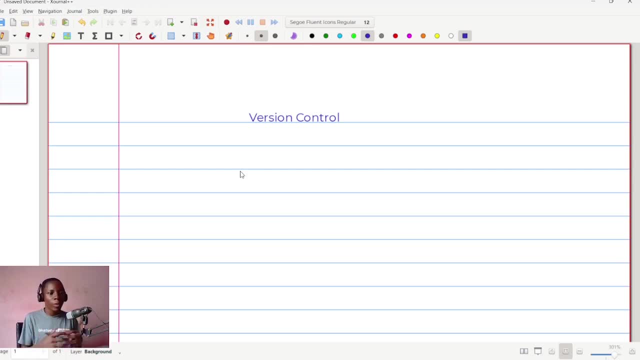 then, when you come to software development, we are looking at how do i control these versions that i have, how do i manage these versions? am i going to be creating, copying and pasting the various source code that i have, the code that i have to make this commentshop? so i'll close box before accepting the correct application method. 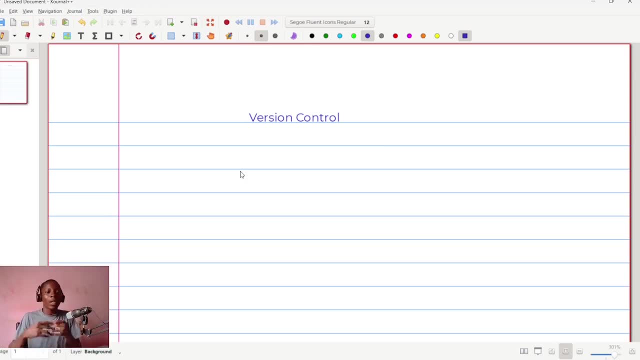 route for this app? am i going to just copy and paste it somewhere else and make changes to it and all so? there are systems that helps us do this easily. they facilitate the process of creating versions that you would not even have to worry yourself about, and these versions are known as: 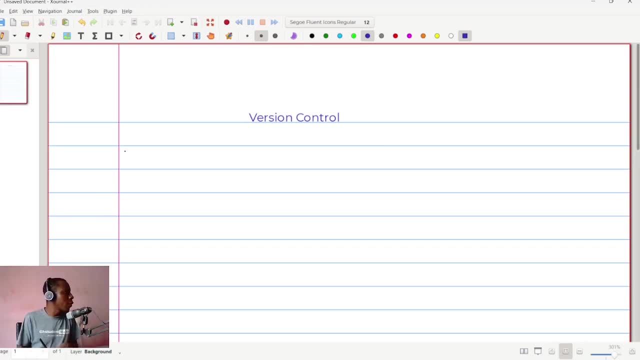 version control system, so you can call them vcs- version control systems, another name that we used to refer to. these are source code management systems. so whether you see vcs or scm, we are referring to basically the same thing, where vcf is version control system and scm is source code. 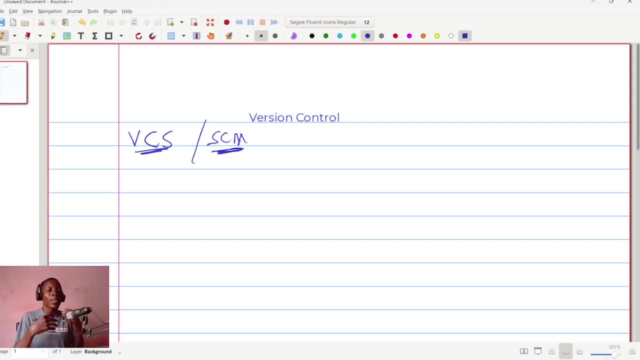 management. so what this means is: this refers to a system, right? remember, we are saying it's a system that allows us to control the versions of our code. so it is going to create a version. so we just have to give particular commands and a version of the source code that we have will be created and we can modify that version. 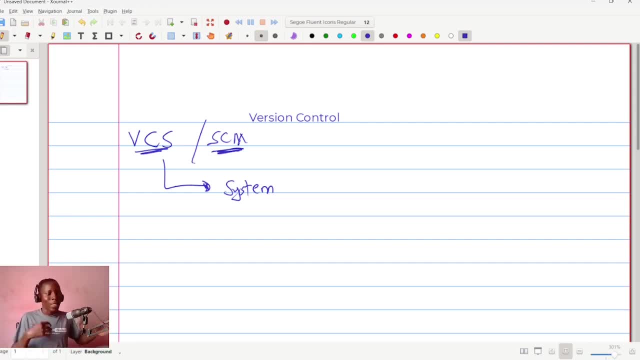 without affecting the original version. just as i explained, if i wanted to create various versions of this, i don't want to destroy this- i still want to have the original version there, then make copies of the original version. so, in the same way, source code control management services or version control systems, allows us to control the various versions. 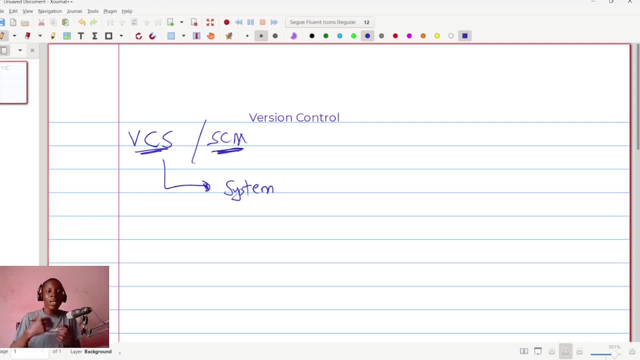 without doing much. we just give it command- and very soon you see some of these commands that we are going to give it to be able to manage this source code or the various versions that we are going to create. so that's essentially what a version control system is, and there are. 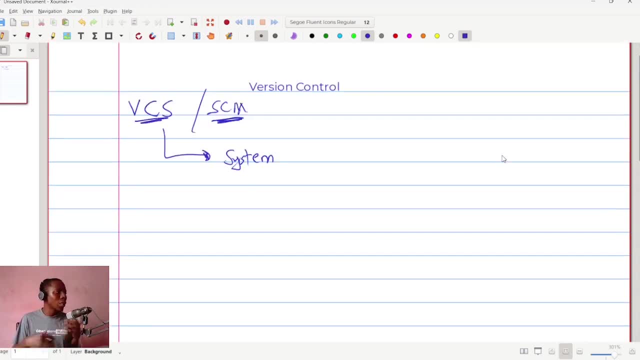 two major types of version control systems. let's quickly get into it then. i mentioned some examples and subsequent videos will dive more into a specific example. so when we talk about version control systems, there are two major types. so the types we have what we call the centralized, the centralized version control system and, as you 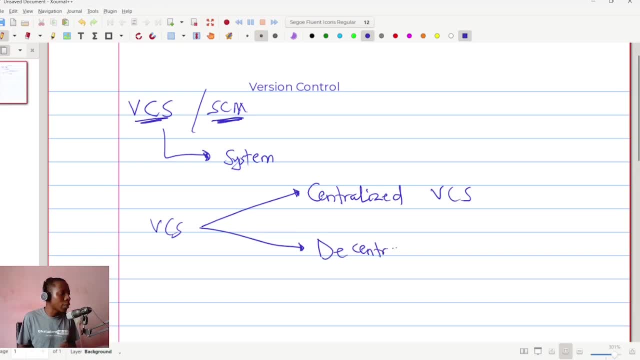 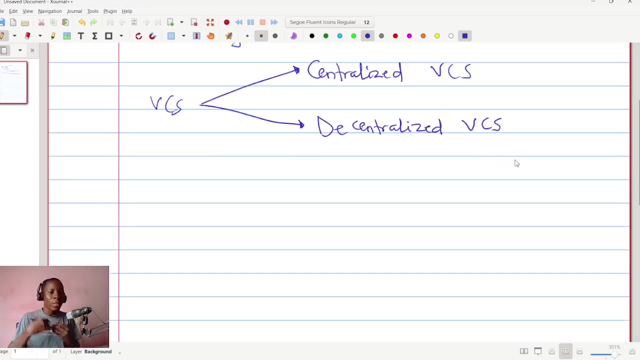 might have guessed the decentralized. so we also have the decentralized version control system. now, to be able to explain this for you to appreciate it, i need to let you on on something, even though we are going to discuss it in subsequent videos. so please, if you don't, 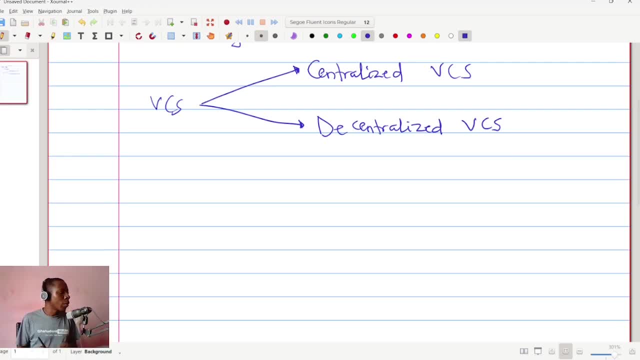 understand it. just take your time. you would appreciate it with them. but when you're working with a version control system, this is what happens. there is a software or a technology, let me call it that way. there is a technology that will take care of the versions right, and that's essentially what the version control system is. but then where? 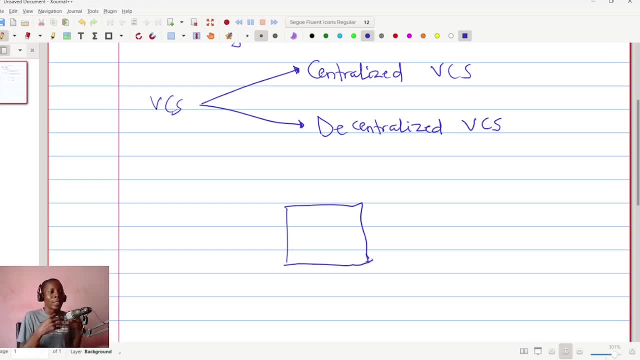 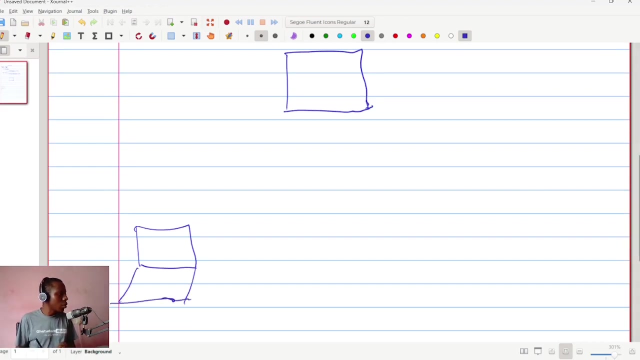 in your workflow as a software developer, is this particular technology installed? is what would differentiate the type? so let's assume that you, the software developer, have your computer here and that technology that you are using, or that technology that allows you to control the systems. okay, so let me mention, let me just use this technology. i will explain it later. 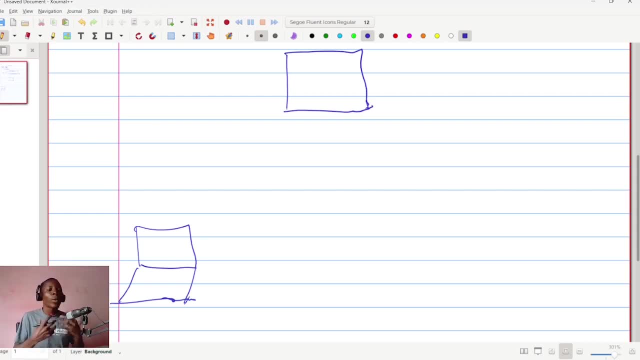 so just keep calm with it. we call something a repository. essentially it is a folder with that source control technology installed in it so that it allows you to control the various versions. so if this is your computer and fortunately or unfortunately, the technology we are talking about is not a source control or the source code management technology is installed on a remote, 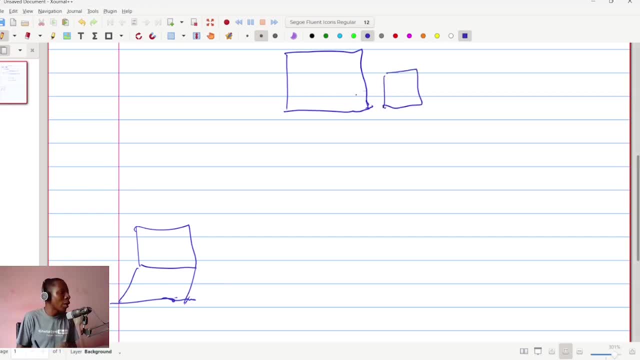 computer on a computer that is not your own computer. so let's say that your repository that you are working with is on this computer. the word i mentioned is repository and i said it's basically a folder with that technology, the version control system, installed in it. all right. 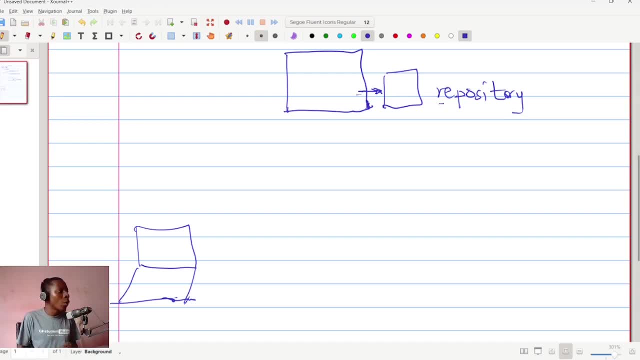 explain it better with time and you would appreciate it. so you have this repository, but the repository is not on your computer, it's somewhere else. that means that a lot of you developers- let's say you work in the same company and you all are going to write some code. you are 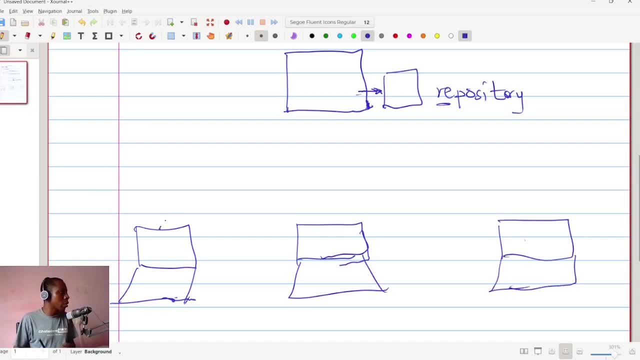 all working on the same project. so this person, who is you, will send his code, all the changes that he's making to this repository, which is not on his computer, it is somewhere far away. they say this other person who is going to do same. send your code there, this person to be doing same in. 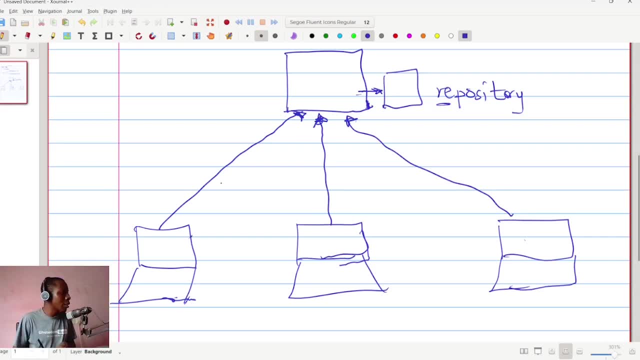 the same way, any updates that come you, the person here- will also have to pull the updates onto your computer. this other person to have to pull any updates onto his computer to be able to work on a new version that has been created. so at any point in time you see that you are pushing to. 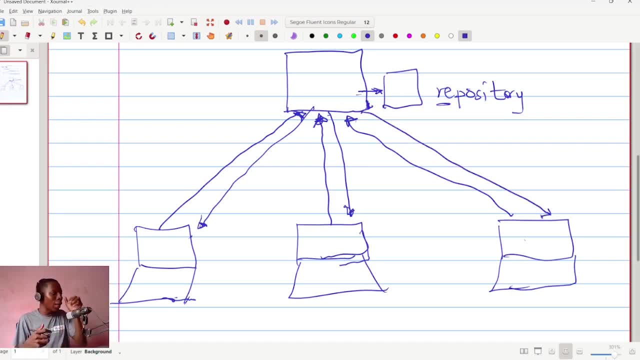 that repository or you are pulling from that repository. if this is the nature of it, then we say you are working on a centralized version control system. the reason why it is centralized is because the repository that we are all pushing and pulling from is a central repository. it's just. 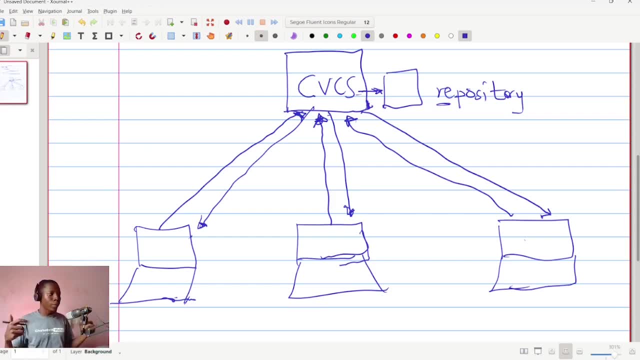 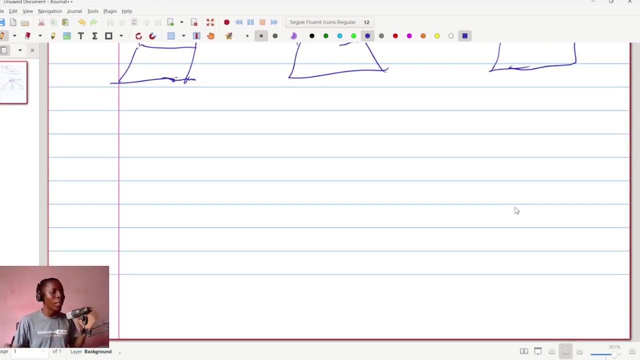 a central repository that we all push and pull from. so, on that note, let's discuss what additional a decentralized- uh, a decentralized- version control system will be. on the other hand, with a decentralized version control system, every one of the software developers would have on their own computer a repository, and we call that a local repository. so now, instead of pushing directly to 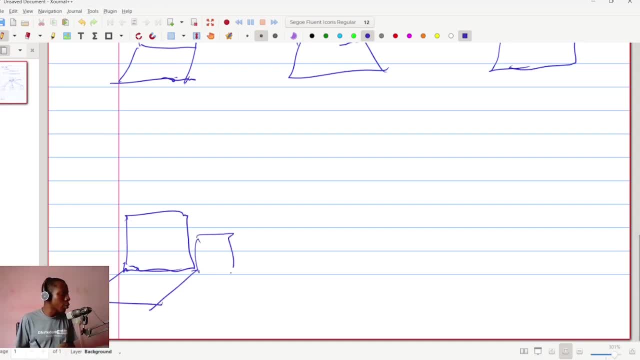 that central repository you are going to have a on your own computer such that when you make you create your versions or you make changes to the code, you push it to your local. this other developer tool will do same. they are able to push the code to their local repository and, the same as this other developer push the code towards.